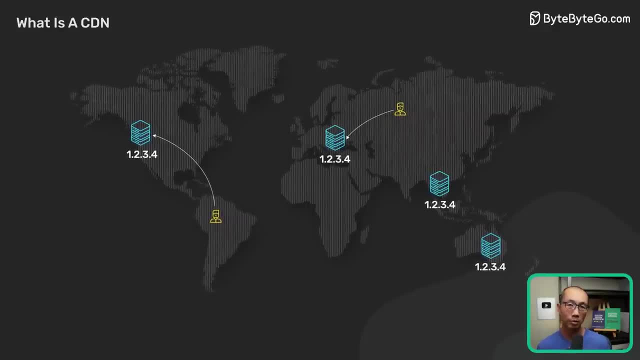 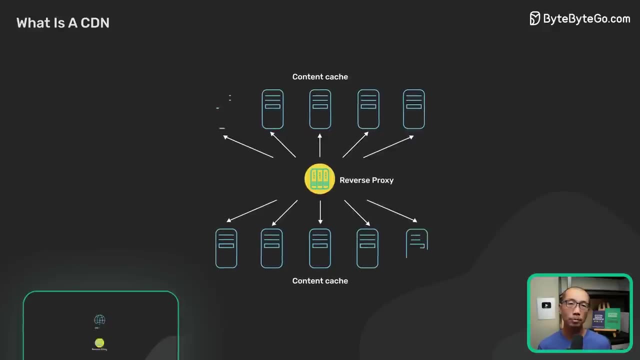 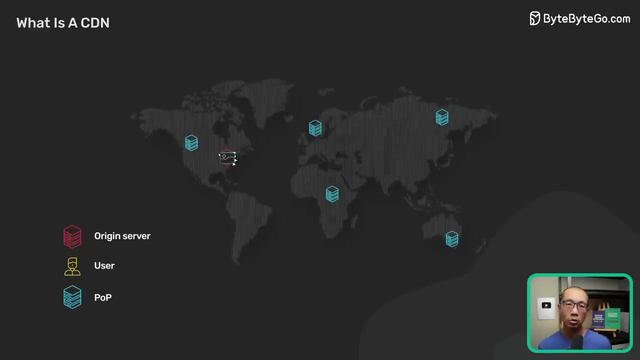 sends the request to the POP that is closest to the requester. Each edge server acts as a reverse proxy with a huge content cache. We talked about reverse proxy in an earlier video. Check out the description if you'd like to learn more. Static contents are cached at the edge server in the content cache. If a piece of content 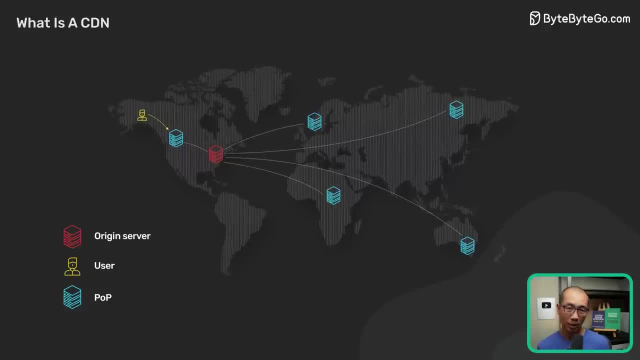 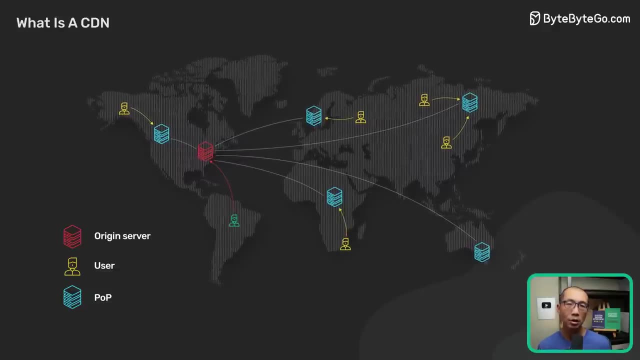 is in the cache, it could be quickly returned to the user, Since the edge server only asks for a copy of the static content from the origin server if it is not in the cache. this greatly reduces the load and bandwidth requirements of the origin server cluster. 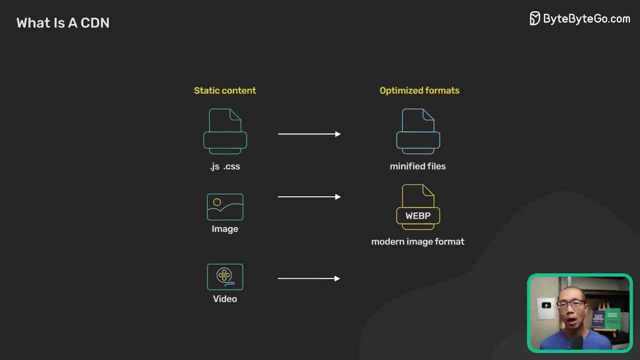 One CDN could also transform static content into more optimized formats. For example, it could minify Javascript bundles on the fly or transform an image file from an old format to a modern one like WebP or AVIF. The edge server also serves a very important role in the modern HTTP stack. All TLS connections. 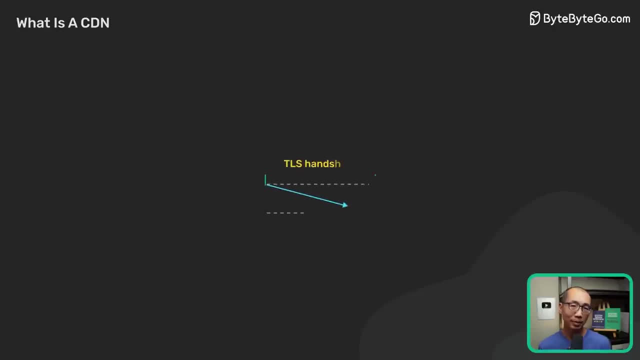 terminate at the edge server. TLS handshakes are expensive. The commonly used TLS versions, such as the TLS server, are very expensive. TLS handshakes are expensive. The commonly used TLS versions, such as the TLS server, are very expensive. 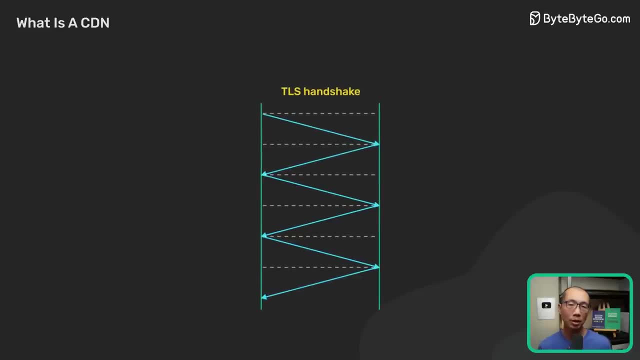 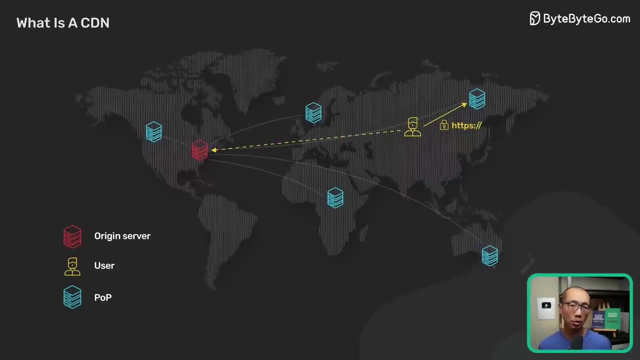 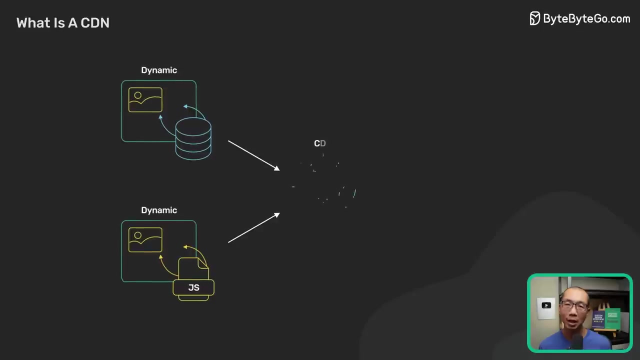 The TLS 1.2 takes several network round trips to establish. By terminating the TLS connection at the edge, it significantly reduces the latency for the user to establish an Encrypted TCP connection. This is one reason why many modern applications send even dynamic, uncacheable HTTP content. 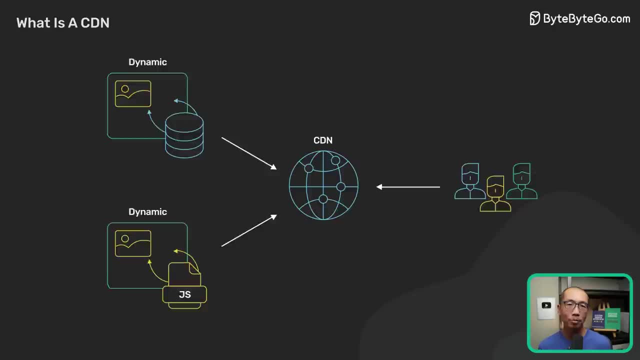 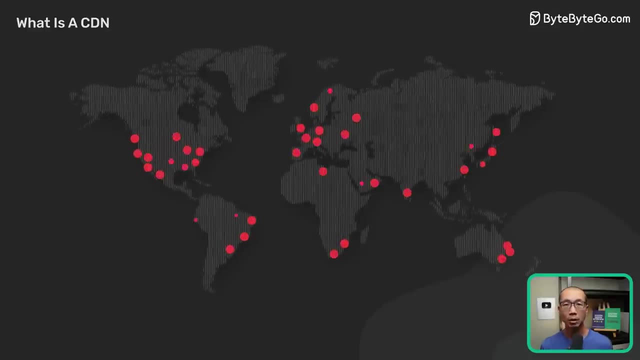 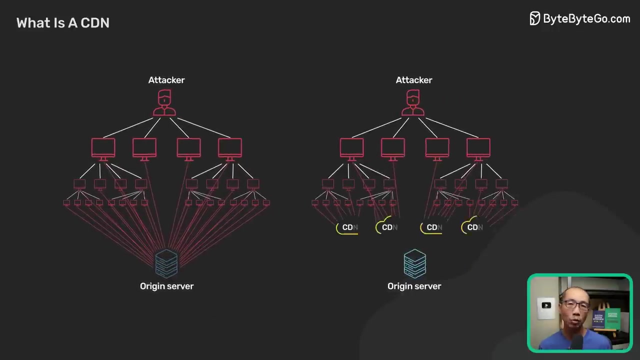 over the CDN. Besides performance, a modern CDN brings two other major benefits. First is security. All modern CDN has huge network connectivity, huge network capacity at the edge. This is the key to providing effective DDoS protection against large-scale attacks, by having a network with capacity much 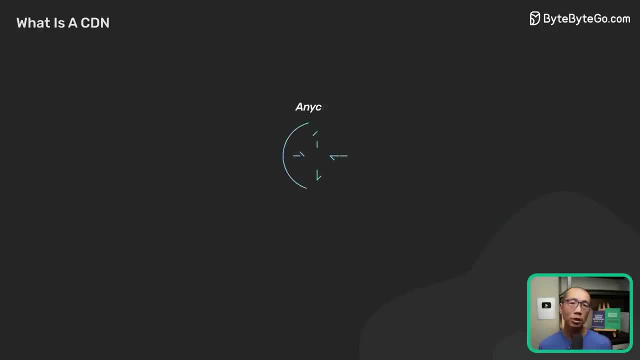 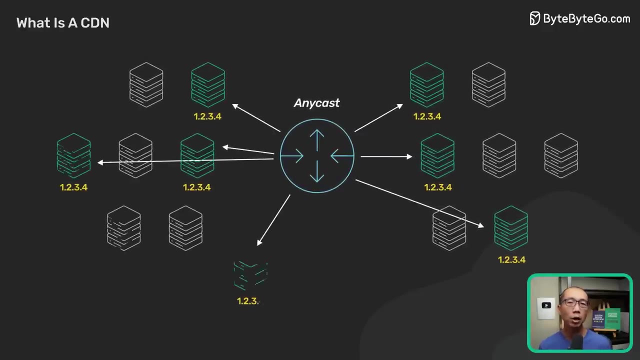 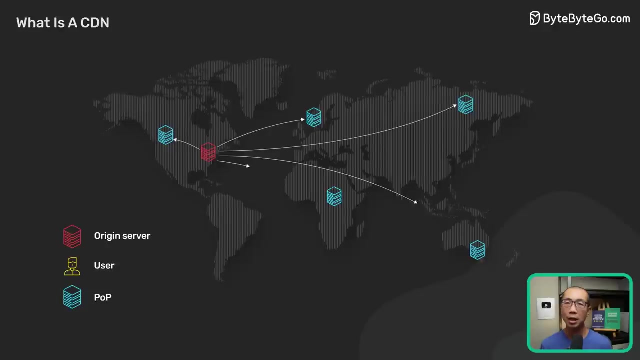 larger than the attackers. This is especially effective with a CDN built on an Anycast network. It allows the CDN to defuse the attack traffic over a huge number of servers. Second, a modern CDN improves availability. A CDN by its very nature is highly distributed By having copies of contents available in many